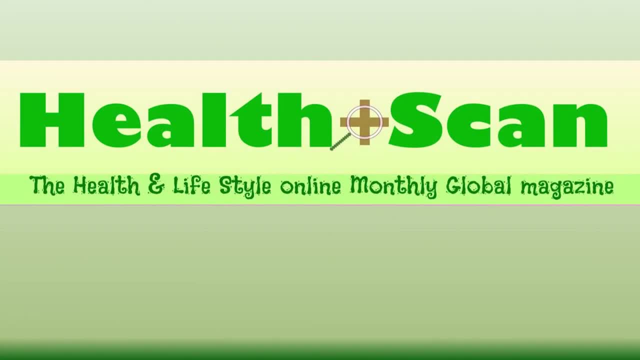 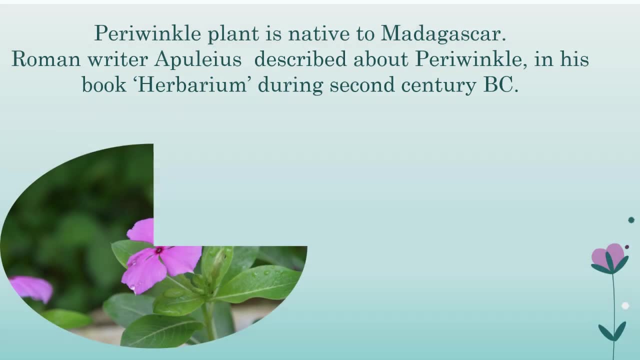 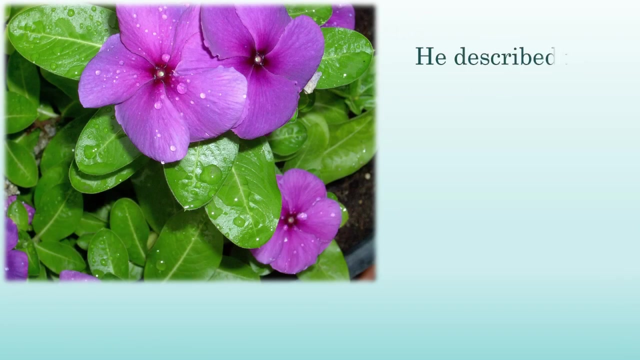 Periwinkle plant is native to Madagascar. Roman writer Apollios described about periwinkle in his book Herbarium during 2nd century BC. He described its virtues against the devil's sickness and demoniacal possessions and against snakes and wild beasts In the Indian Ayurveda. 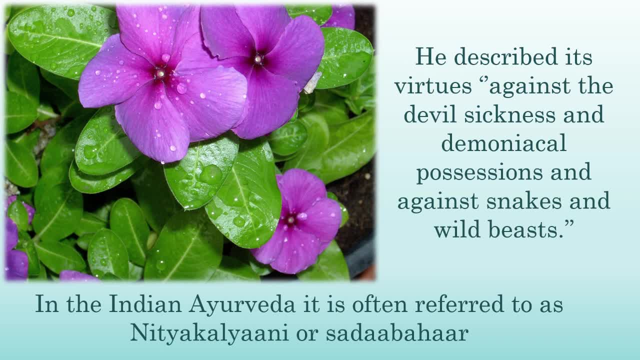 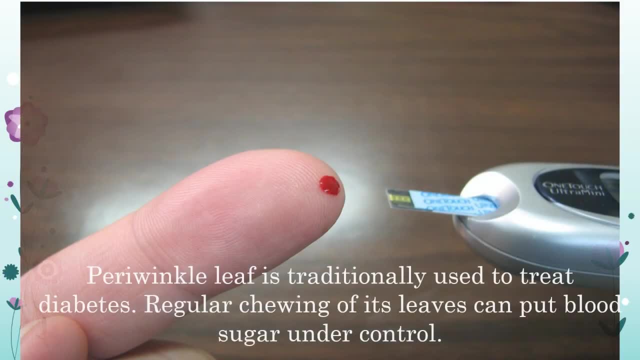 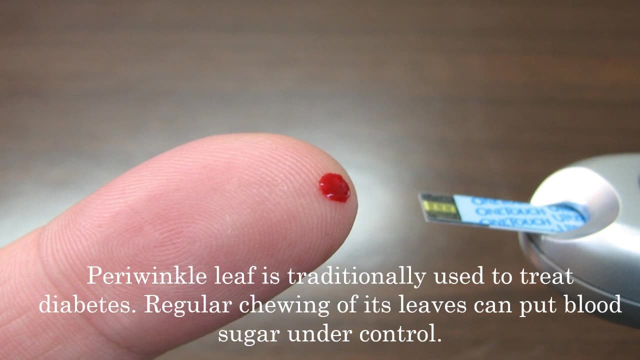 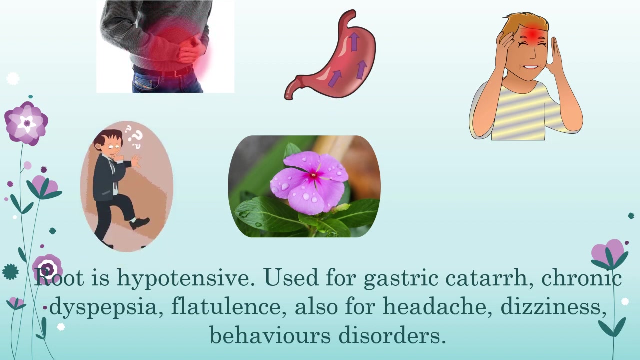 it is often referred to as Nithya Kalyani or Sada Bahar. Traditional Medical Uses: Periwinkle leaf is traditionally used to treat diabetes. Regular chewing of its leaves can put blood sugar under control. It is high potency used for gastric catarrh, chronic dyspepsia, flatulence, also for headache. 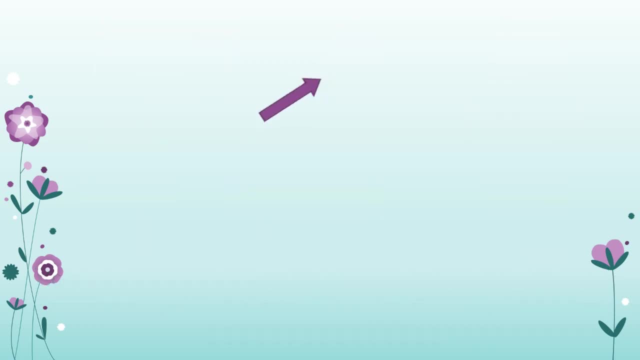 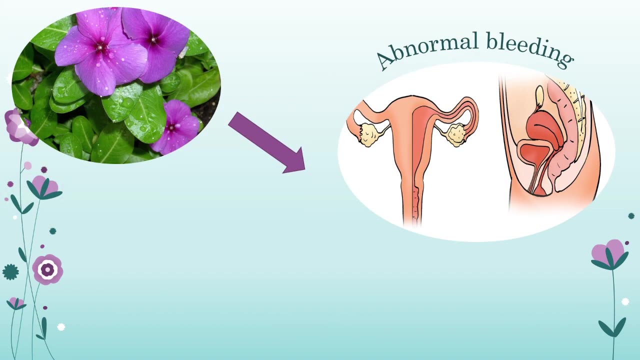 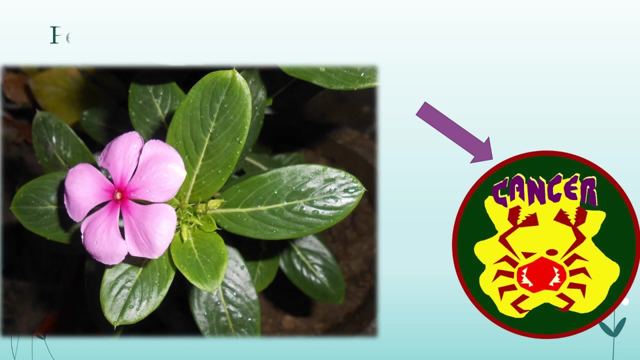 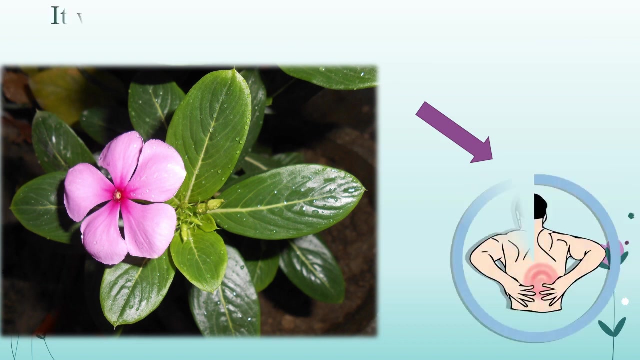 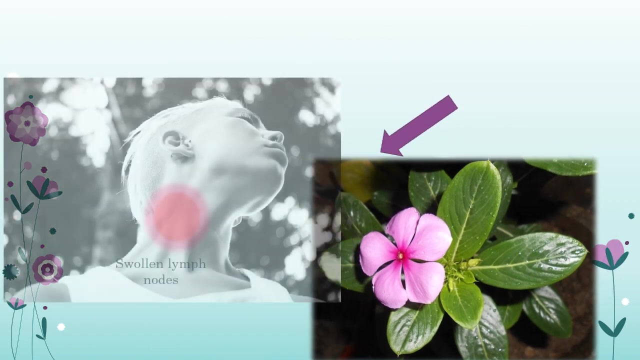 dizziness behaviour disorders. Periwinkle is known for its potential to curb bleeding. Periwinkle is used for Menorrhagia and Leukorrhoea. Periwinkle is used to treat some types of cancer. It works as antispasmodic. Traditionally, leaves are used in treating Hodgkin's disease. 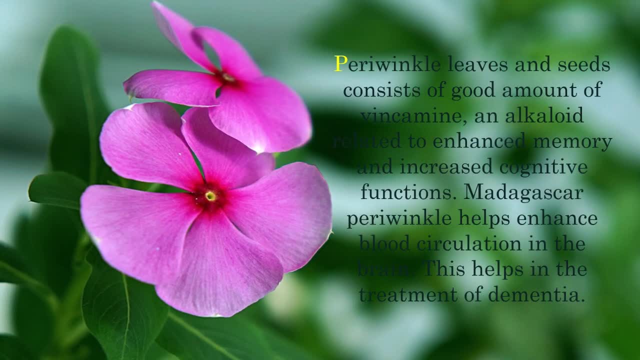 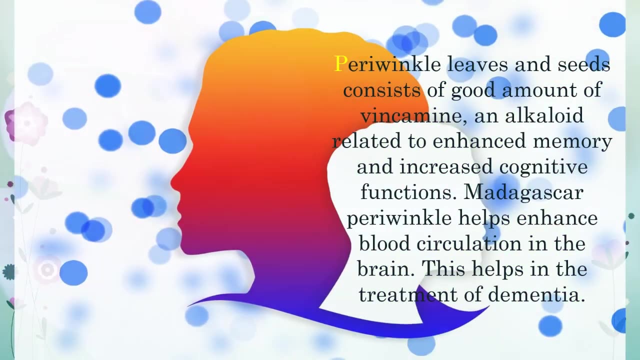 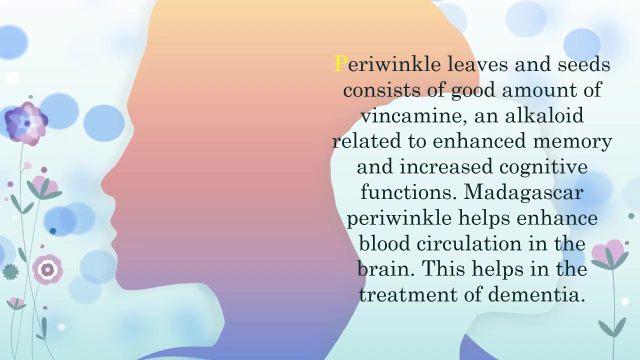 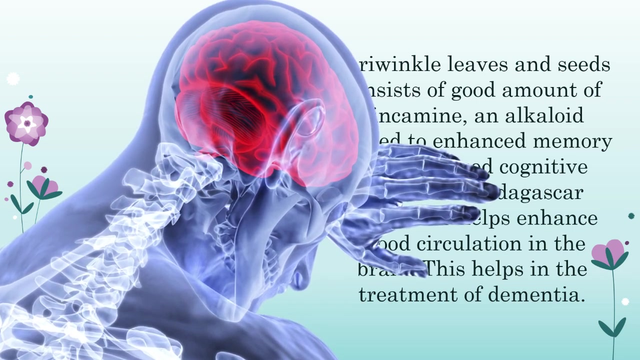 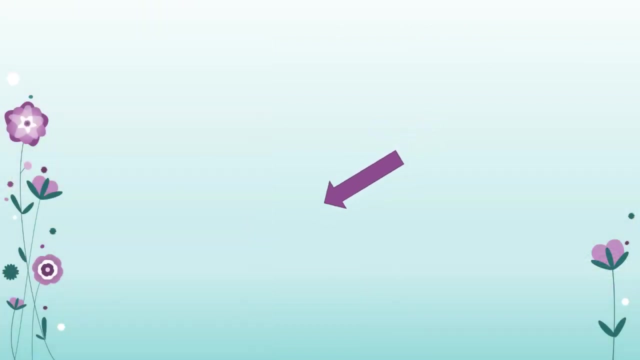 Periwinkle leaves and seeds consist of good amount of vincaimin, an alkaloid related to enhanced memory and increased cognitive functions. Madagascar Periwinkle helps enhance blood circulation in the brain. This helps in the treatment of dementia. It is also used in wound healing. It contains alkaloid Recipain, which is effective for